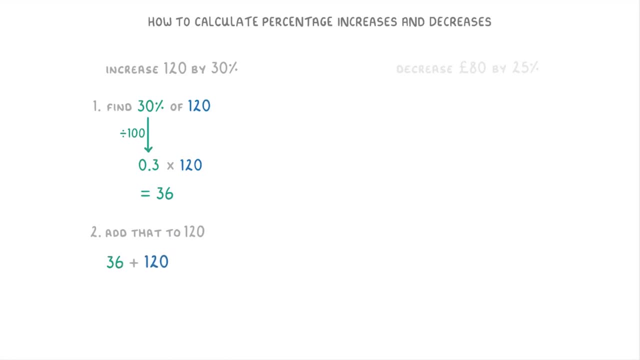 36 to the original of 120, to get a total of 156, which would be our final answer. For this next one, we need to decrease 80 pounds by 25%. So, similar to before, we first need to find out what 25% of 80 pounds is And then, because it's a decrease this time, 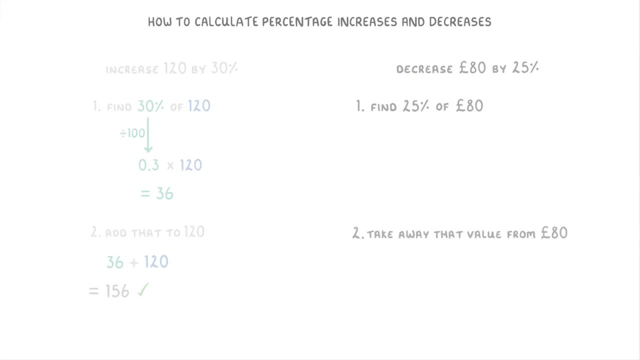 we have to take that value away from the 80 pounds, So to get 25% of 80 pounds. we're just going to convert 25% to 0.25 and multiply by 80 to find that it's 20 pounds. Then we 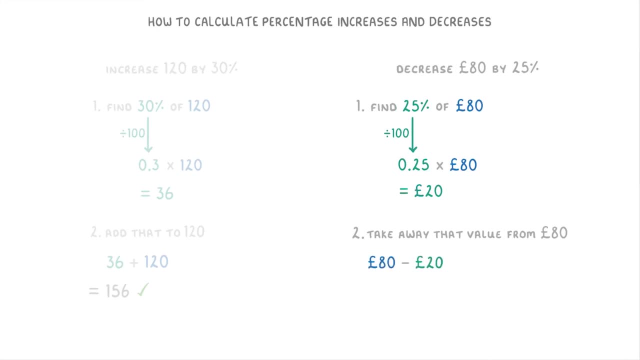 just take that 20 pounds away from the original 80 pounds to get a new price of 60 pounds. Let's have a go at another one with some context this time. Charlie wants to buy some new headphones which normally cost 142 pounds. If he uses 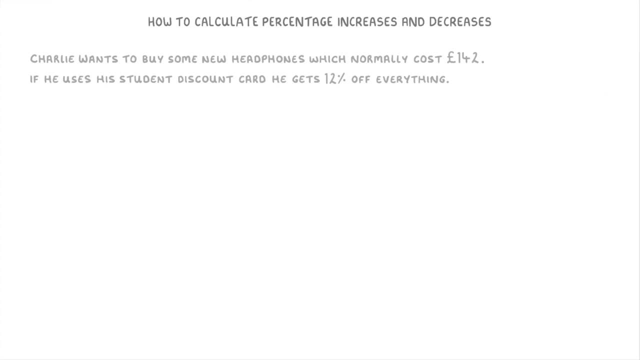 his student discount code, he'll be able to buy a new pair of headphones, which normally cost 12% of everything. How much would he have to pay for the headphones if he used his student discount card? So in this question there are really just three important bits that we need to notice. 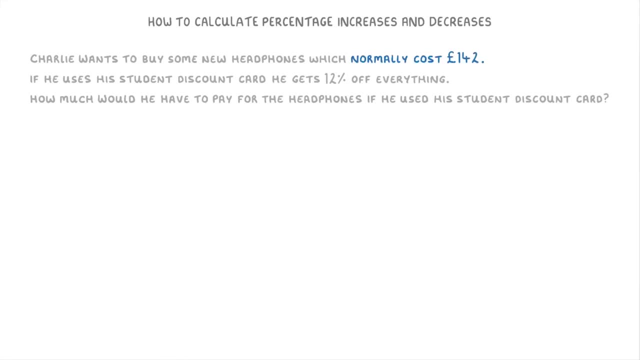 The fact that the normal cost is 142 pounds, the fact that it's a discount, so we're reducing the price, and that the size of the discount is 12%. So if we take these three points together, we're really being asked. 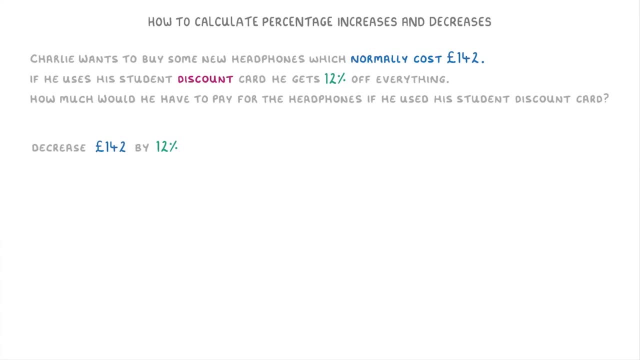 to decrease 142 pounds by 12%, And this means that the first thing we need to do is convert 12% to 0.12 and multiply it by 142 pounds to find that the 12% is worth 17 pounds, and 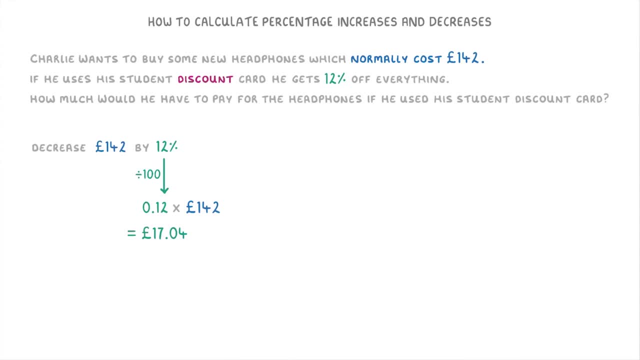 four pence. Then we can subtract that discount from the original price of 142 to get the discounted price of 124 pounds 96.. Okay, Next up, we need to look at the other technique that we can use, which is called the multiplier method. The trick with this method is to think of the original number. 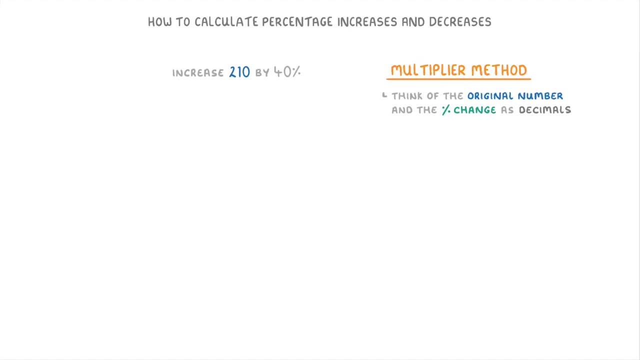 and the percentage change, both as decimals. So in this question, 210 is the original number which we can think of as worth 100% or 1, because it's the entire original number, whereas the 40% is the percentage change. and 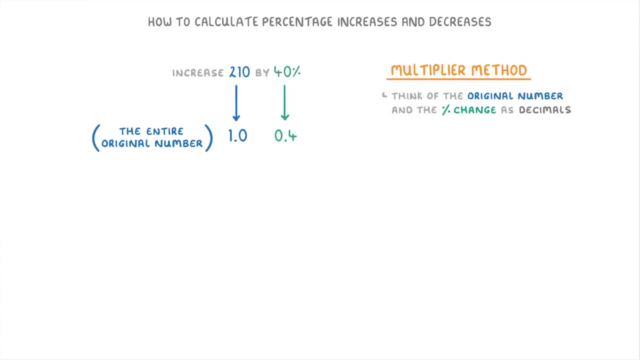 is equivalent to 30.. to 0.4, because to get percentages to decimals we just divide them by 100.. So for a percentage increase question where we're basically trying to find 210 plus 40%, we can use these decimals instead and think of it as trying to find 1 plus 0.4.. So we just 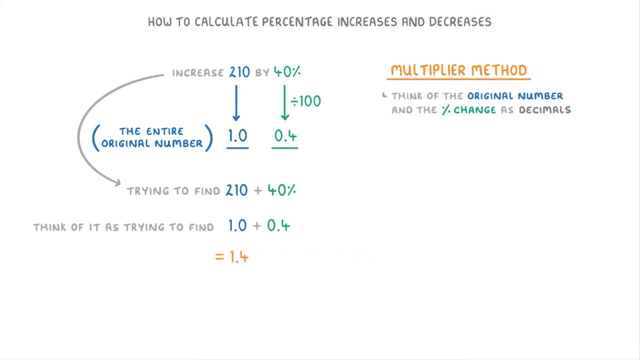 add them together to get 1.4, which we call our multiplier, and then we multiply that 1.4 by the original 210, to get an answer of 294.. I know this method is kind of confusing at first, so let's have a go at another couple questions. 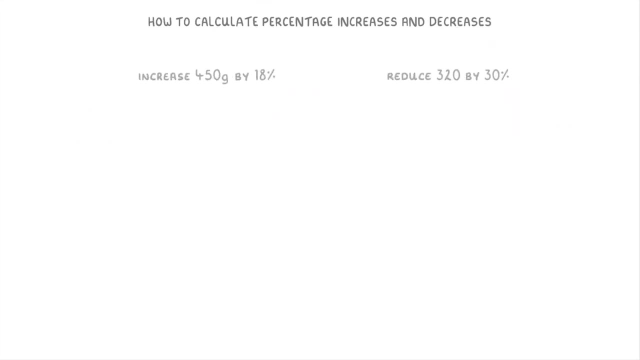 In this first one we're trying to increase 450 grams by 18%. So we think of the 450 grams as 1, because it's the original number, and then think of the 18% as 0.18.. Then, because the question says increase, we add those together to get 1.18,. 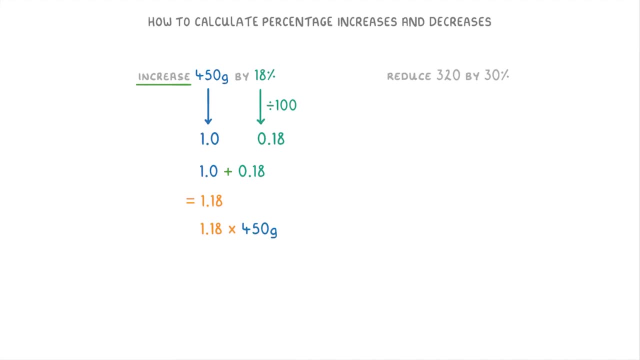 and multiply the 1.18 by 450 to get the new mass of 531 grams. For this second one, we need to reduce or decrease 320 by 30%. So this time we still think of 320 as 1, and write the 30% as 0.3,. 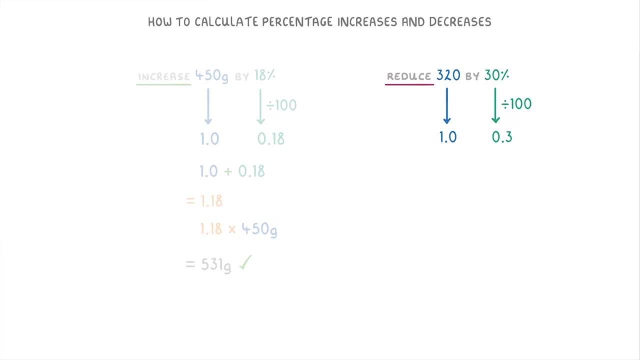 but because we're reducing or decreasing, this time we're to do 1 minus 0.3 to get 0.7 as our multiplier. Then we just multiply 320 by 0.7 to get our new value of 224.. 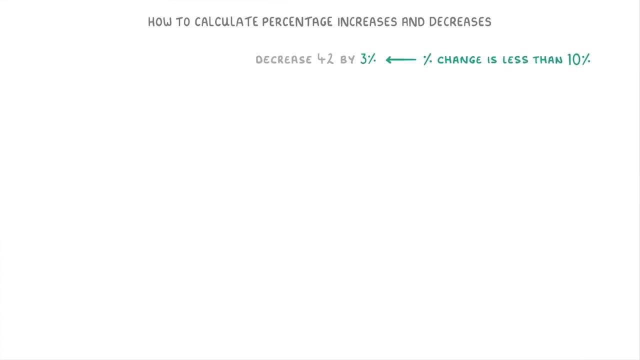 Now, one thing to watch out for with these is when the percentage change is less than 10%, like here, where we're trying to decrease 42 by 30%. 3% is equivalent to 0.03.. So we'd have to do 1 minus 0.03 to give us 0.97 as our multiplier.